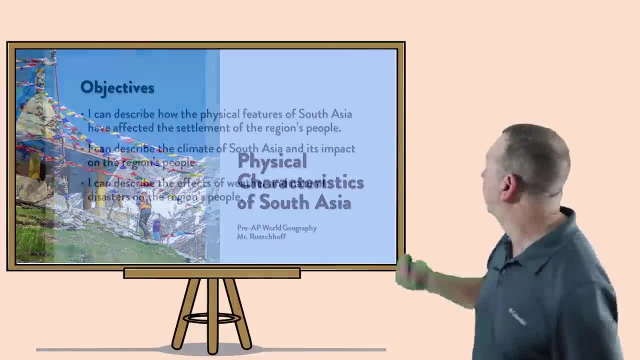 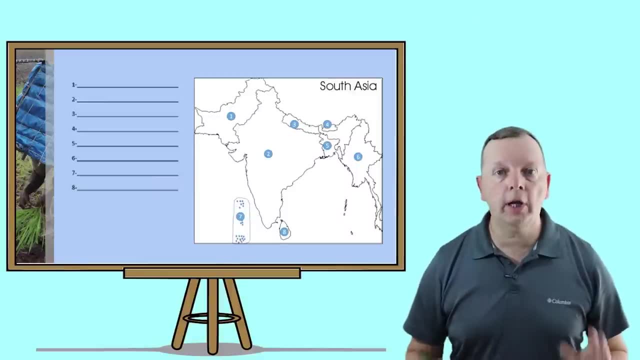 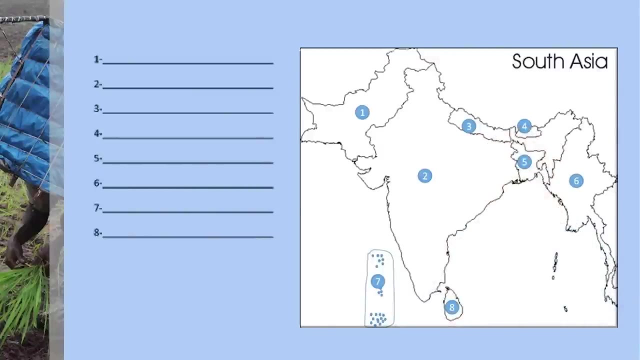 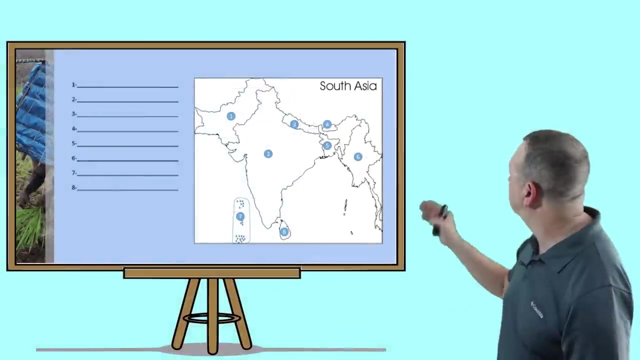 by looking at its physical characteristics. And here are our objectives we're going to be following. Alright, let's go ahead and enjoy. And number eight is Sri Lankan. If you look at the shape of Sri Lanka, you'll understand the reason why it has earned the nickname. 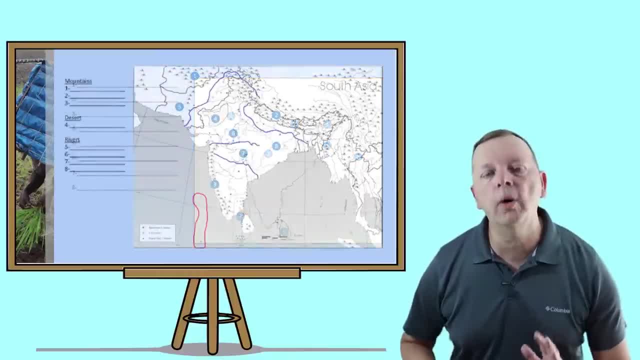 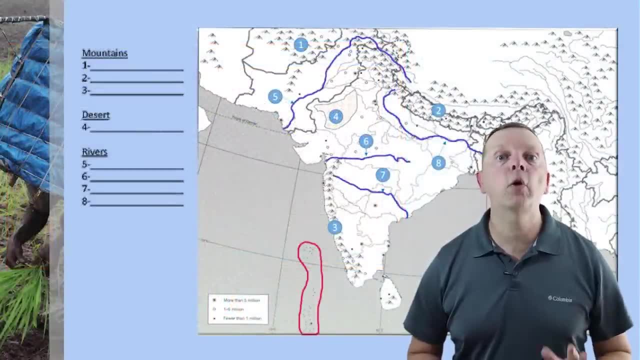 the Teardrop of India, And there are a total of eight different physical features we're going to talk about. There are three mountain ranges, there is one desert and then there are four rivers. So first of all, let's look at those mountains. 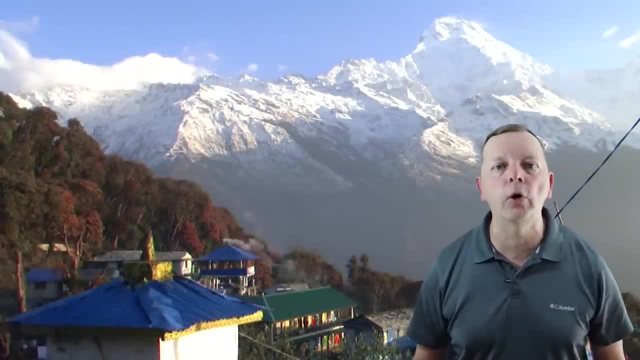 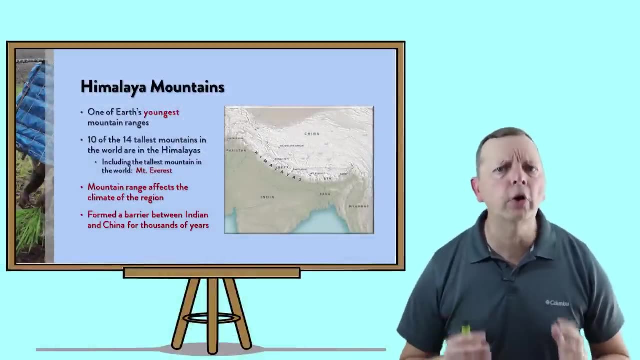 And when we talk about mountains, it is in South Asia. we have the largest mountains in the world, which are the Himalayas. They also are the youngest mountains in the world. Remember, younger mountains actually tend to be taller because they haven't been eroded. 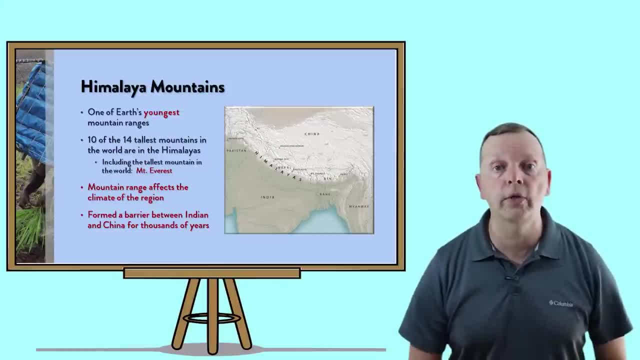 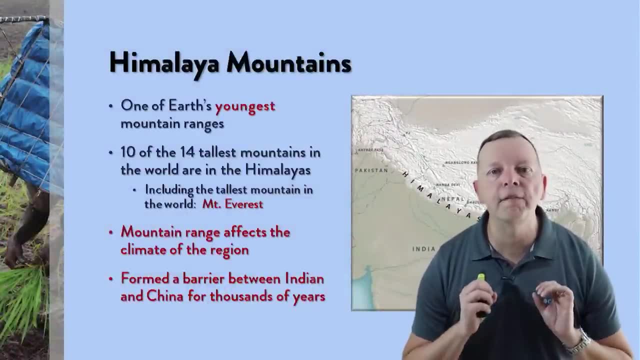 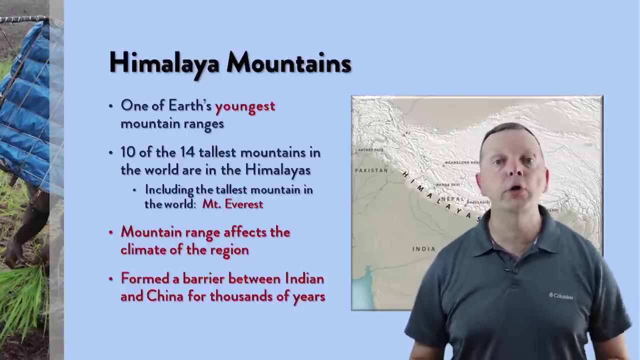 Remember the discussion we had about the Appalachians and the Rockies in North America. Now it is in the Himalayas that we have the tallest mountains in the world. In fact, of the 14 tallest mountains in the world, 10 of these are found in the Himalayas, to include Mount Everest. 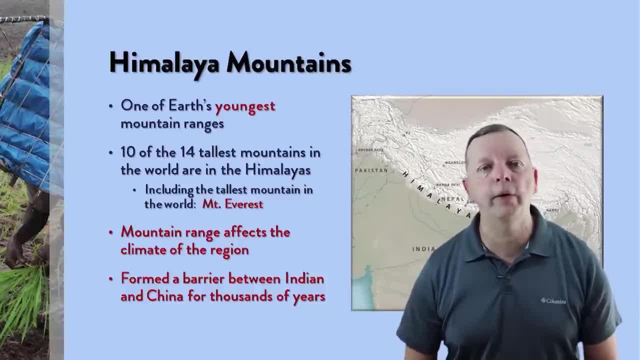 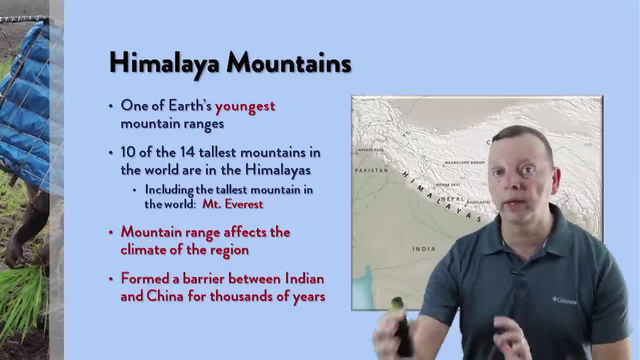 which is the tallest mountain in the world. Now, the Himalayas do two very important things. First of all, they really impact the climate of not only the people in South Asia, but also East Asia. We'll talk about that when we talk about China in the next unit. 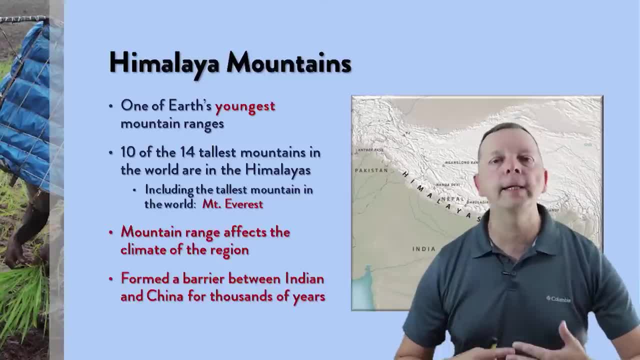 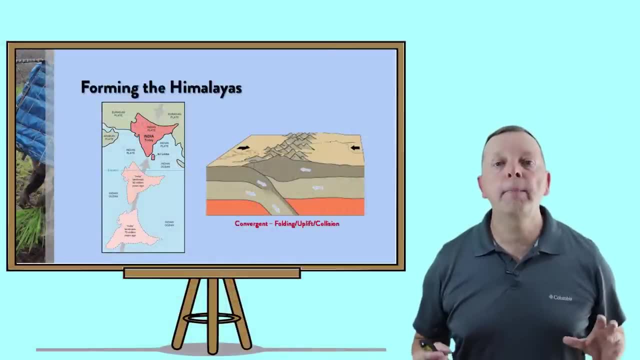 And then also for thousands of years, the Himalayas were a barrier between the people in China and the people in India. The Himalayas are a product of cultural folding And this caused between 50 million years ago and even going on today, of the Indian subcontinent actually. 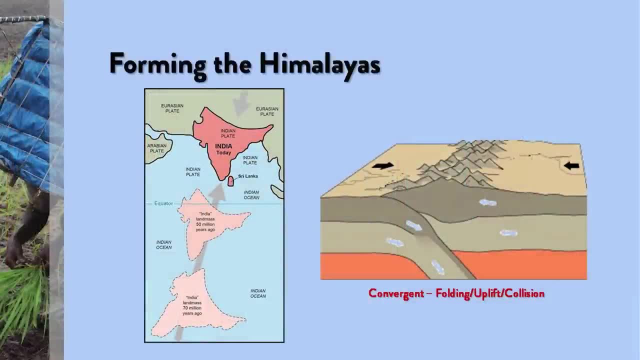 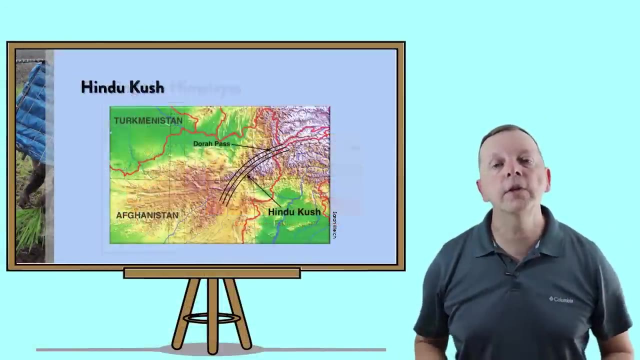 crashing into the Asian continent. In fact, this process continues on today as that subcontinent of India continues moving northward, And this is the reason why Mount Everest continues to grow an eighth of an inch every year. The second mountain range we're going to talk about is the Hindu Kush. 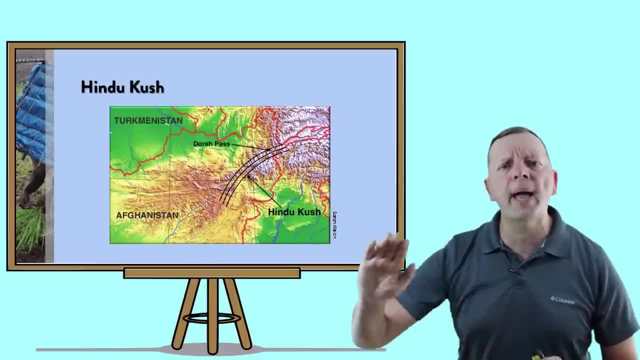 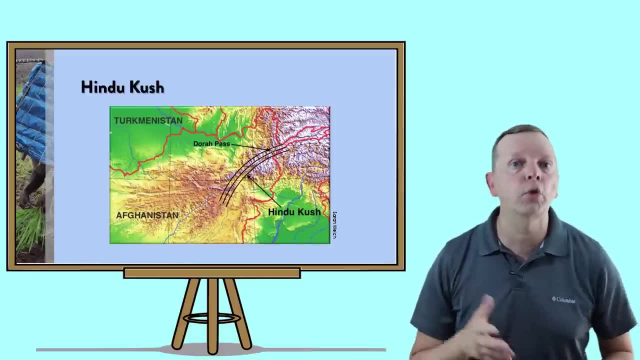 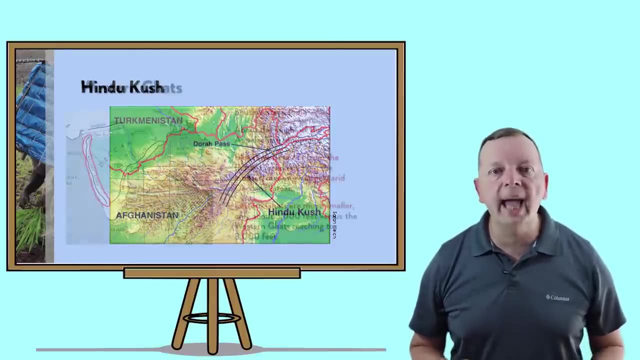 We talked about this during Central Asia. These are the mountains that run from Pakistan down into the central portion of Afghanistan. Now, these also are Our very tall mountains are over 20,000 feet, But what are not very tall are our third mountain range, which are the Western Ghats. 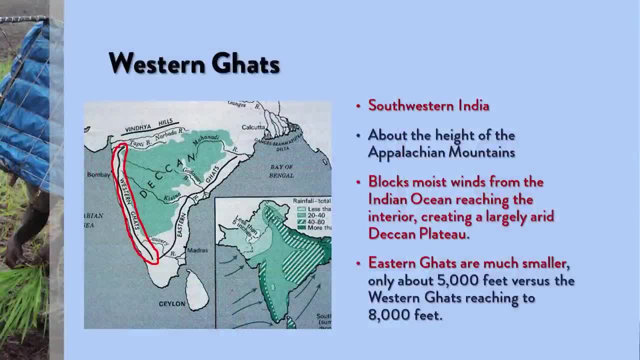 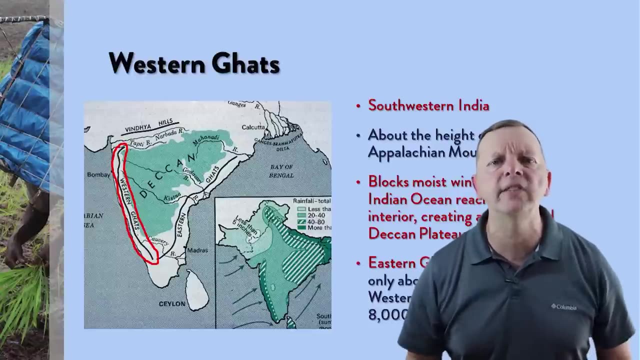 We find our Western Ghats are in the southwestern coast of India And they only are about 8,000 feet, but they still have an impact upon the climate because they help blocks the moisture from the Indian Ocean going into the interior, creating a semi-arid region known as the Deccan Plateau. 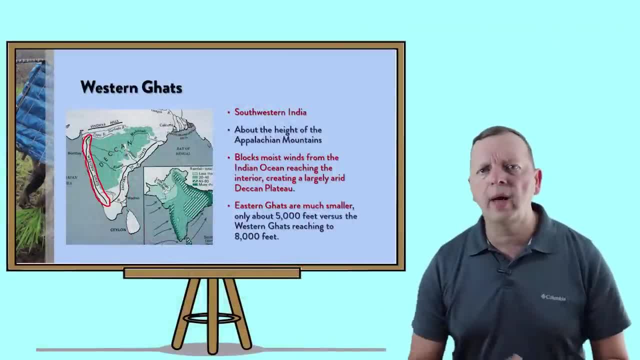 Now there is another Mountain range that we don't have on your map, but I'll talk about very quickly, which is your Eastern Ghats. The Eastern Ghats also runs along the coastline, but along the eastern coastline of India, But these only are about 5,000 feet in height. 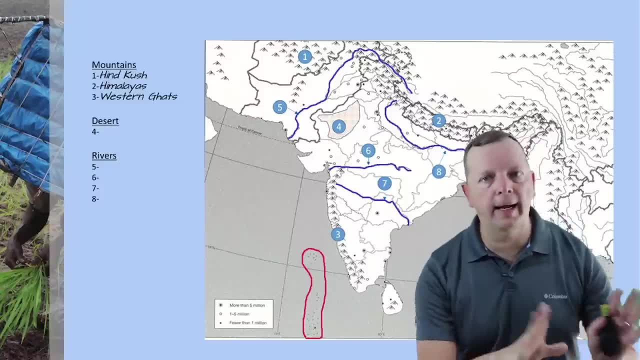 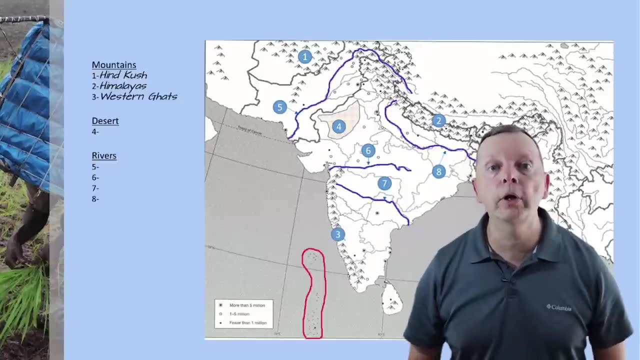 All right. So on our map number one, we have the Hindu Kush, And yeah, I skipped a U there. Number two is our Himalayas, And number three are our Western Ghats. Now what we're going to do is we're going to talk about the deserts. 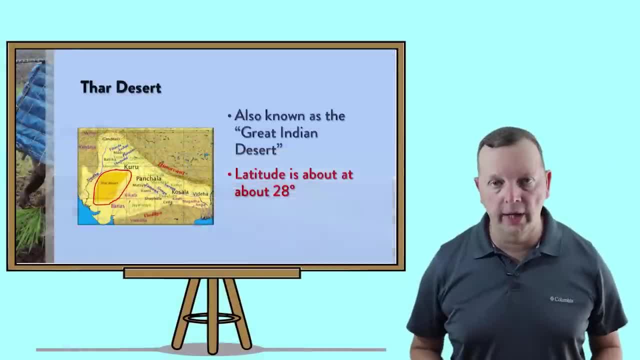 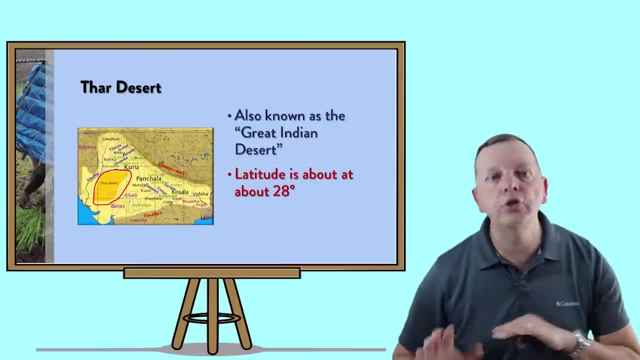 And the desert we're talking about is the Thar Desert, which is also known as the Great Indian Desert, And it is found in the northwest portion of India, just as you're getting ready to go into Pakistan. Now, there are two different reasons for its creation. 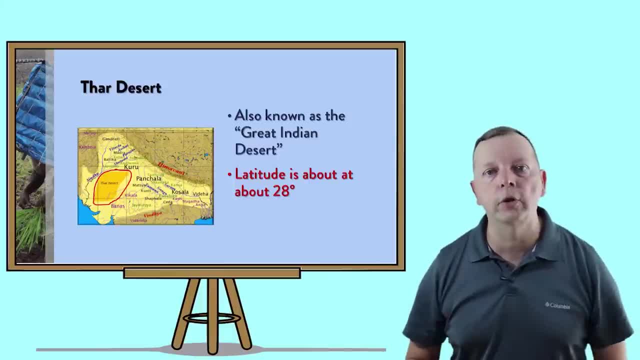 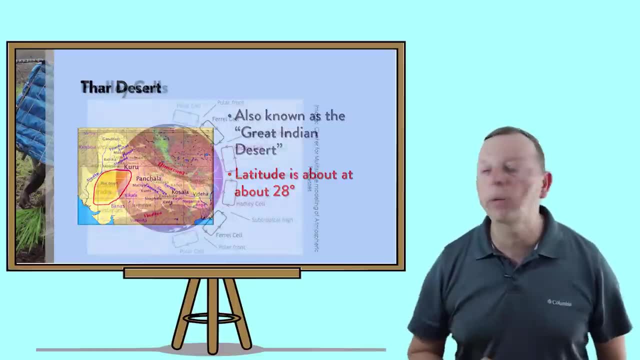 First of all, there's a rain shadow effect of the Himalayas and the other mountains that are around here. Also, it is due to the fact that it's at 28 degrees latitude, And remember when we're talking about the Hadley Cells. 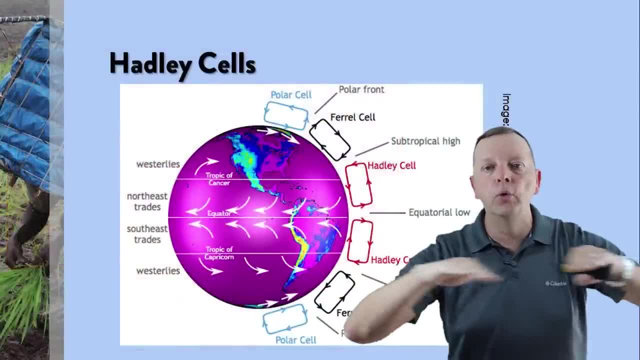 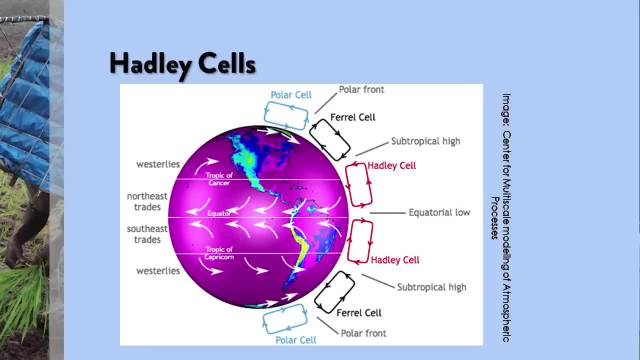 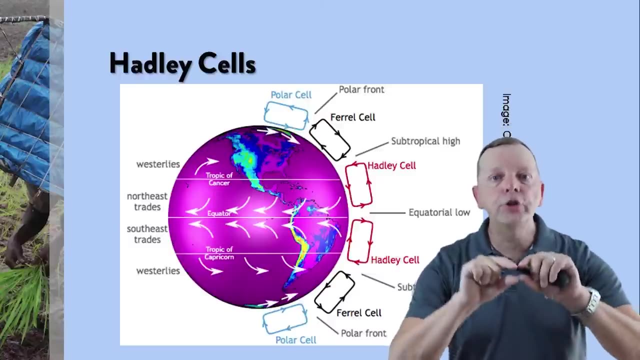 what we know about. At 30 degrees latitude, both north and south latitude, around the world you have these dry high-pressure cells that basically have dry air coming down and pushing moisture away. This is the reason why the largest deserts in the world generally are along 30 degrees. 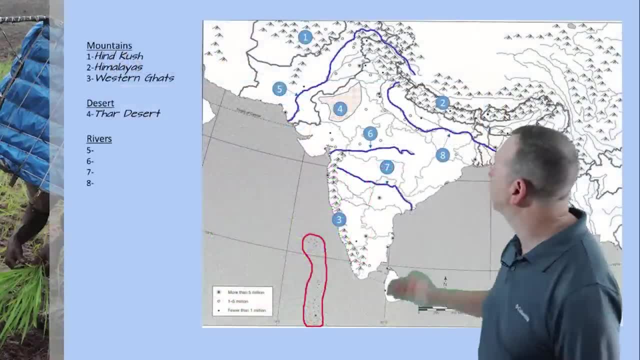 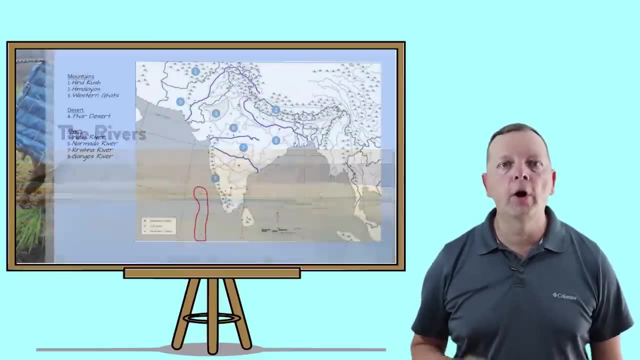 And that is the case we see here with the Thar Desert, which is number four on your map. And then we have some rivers. There's four rivers. we're going to talk about Indus River, which is number five, that runs through Pakistan. 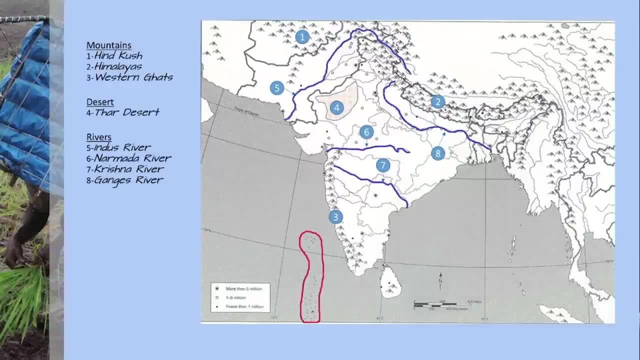 There is number eight, which is the Ganges River that runs through the northeastern portion of India, down through the delta that goes into Bangladesh, And then we have the Narmada River, which is number six, which is just to the north of the Deccan Plateau. 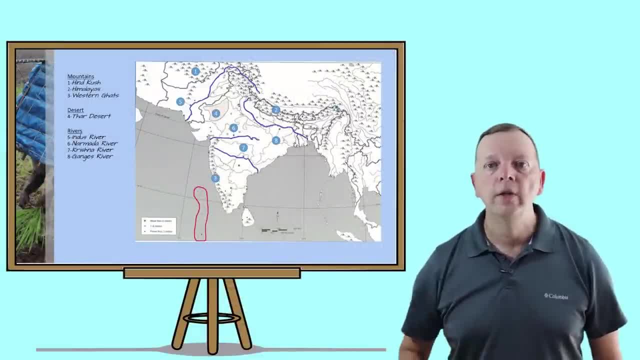 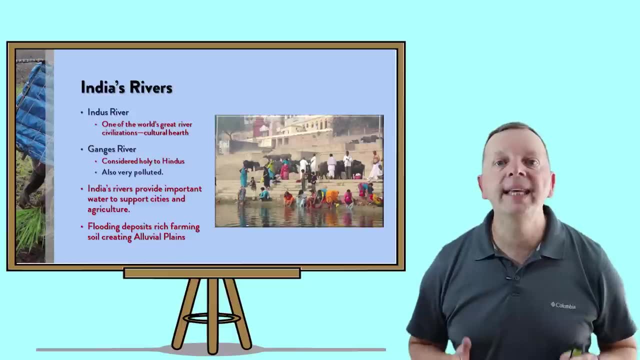 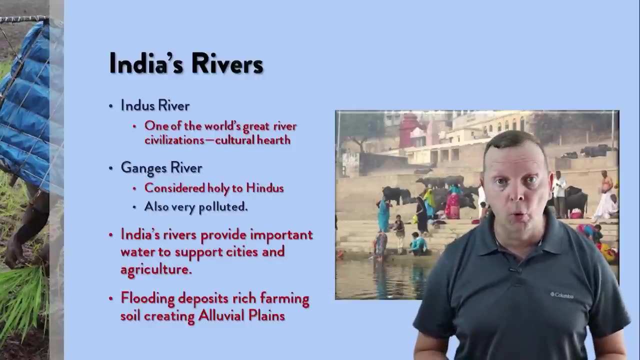 And then we have the Krishna River, number seven- that goes through the Deccan Plateau. Of these, the two most important rivers to know are the Indus River and the Ganges River. The Indus River is important because it is the third of the river civilizations. we've talked about this course. 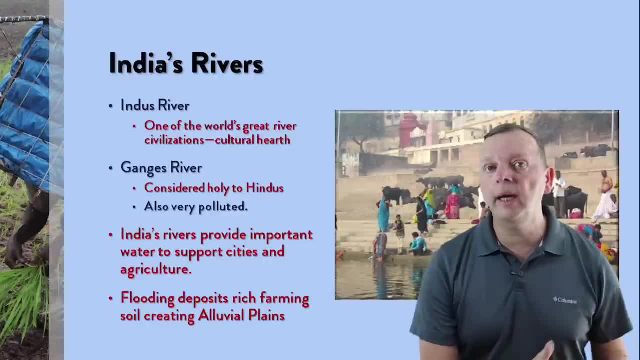 Our first two we talked about, remember, was the Mesopotamia, which is along the Euphrates and the Tigris in the Middle East, and then, of course, there is the ancient Egypt, which has the Nile. 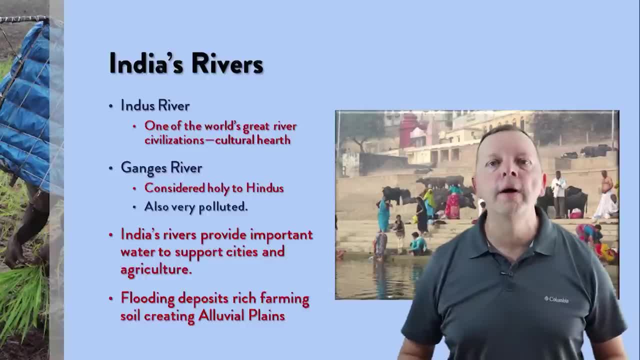 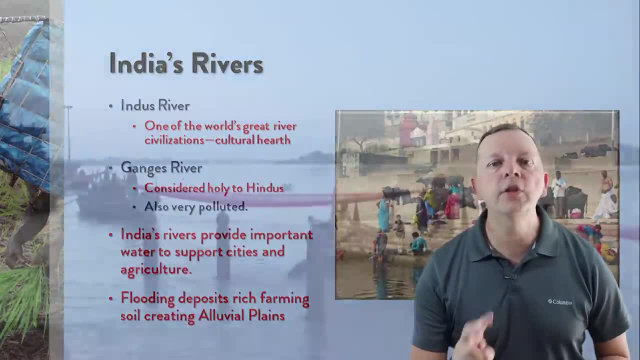 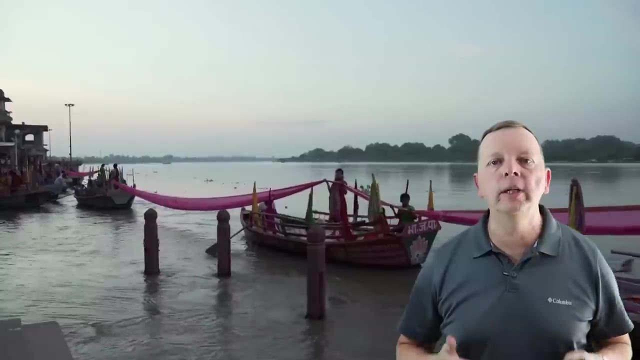 It is along the Indus River that the culture of the people in South Asia actually originated. It is the cultural heart of South Asia. The second river is the Ganges River, And the reason why the Ganges River is important is because it is considered sacred or holy to Hindus. 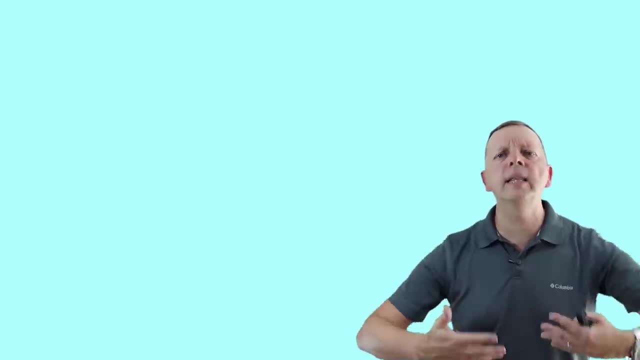 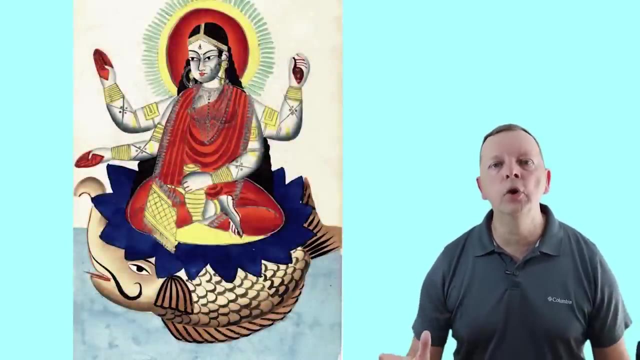 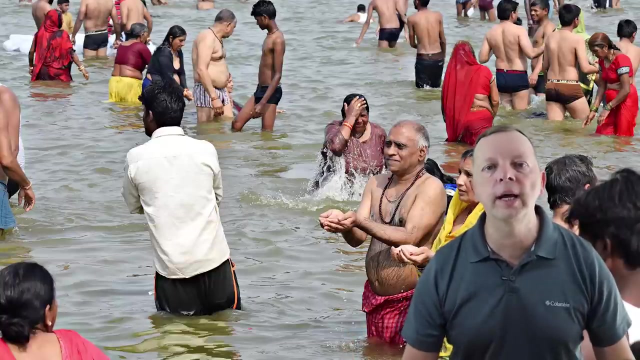 And the reason why it's considered sacred is because it is in the Ganges River that you have the goddess Ganga, And it is said that if you're a Hindu, if you go and bathe in the Ganges River, the goddess Ganga will help absolve your sins and have you move one step more. 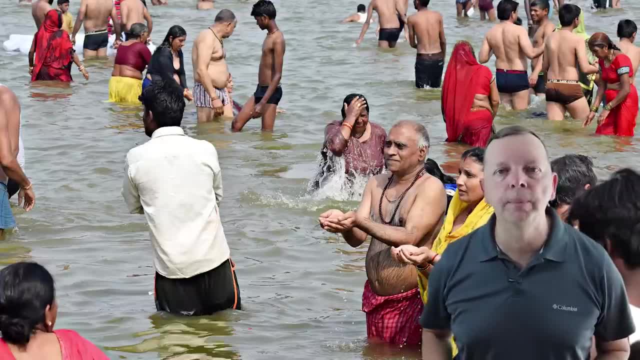 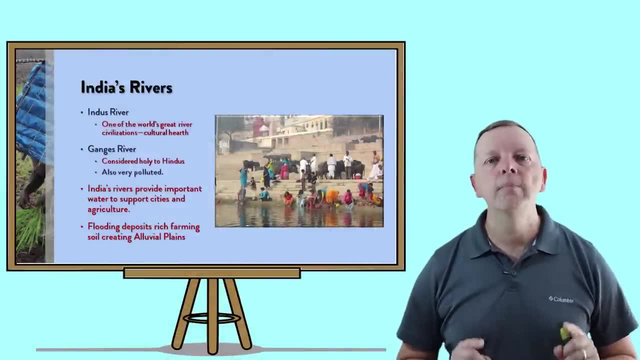 towards Moshka, which we'll talk about when we talk about Hinduism. Now, if this is supposed to wash away your sins, the irony is is that Ganges River is the sixth most polluted river in the world. In fact, in some of the areas, actually have 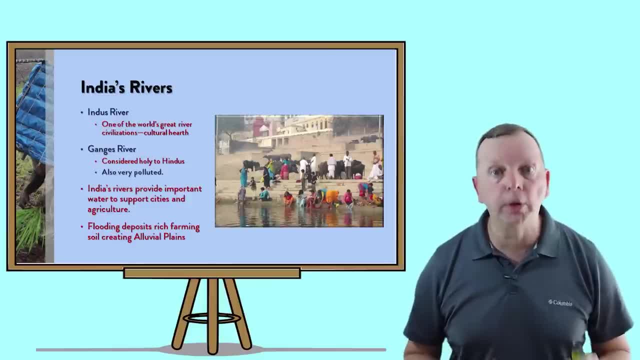 the highest amount of cancer due to the pollution of the Ganges River. Now, these rivers, whether it's these two or also the Narmada and the Krishna, which we talked about before- these are important because they provide water to cities and they provide lands for agriculture. 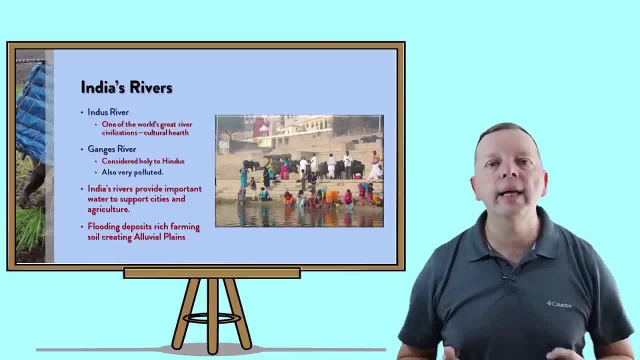 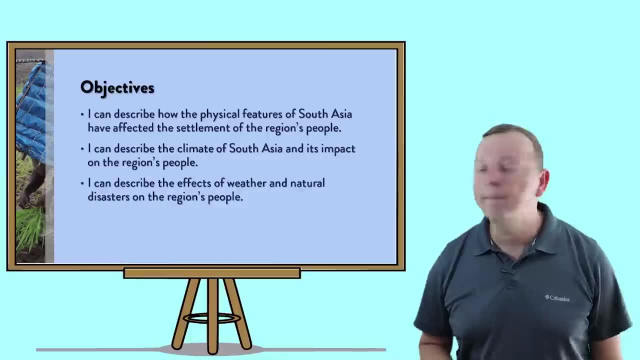 Additionally, whenever you have flooding, it actually allows for very fertile soils to be deposited, known as alluvial plains. All right, So we talked about those physical features that are important to the settlement of South Asia. Now what we're going to do is we're going to talk about the climate and we're going. 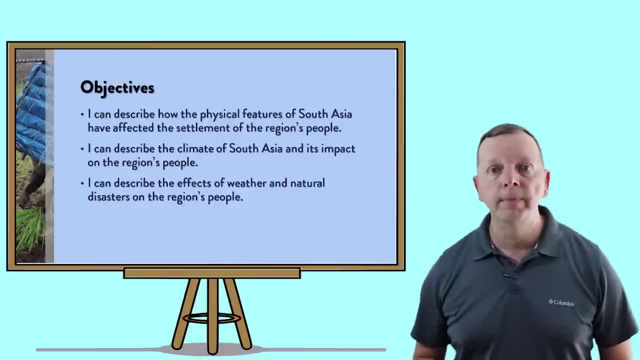 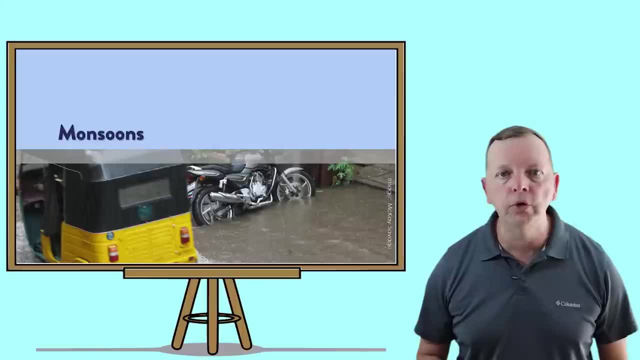 to talk about the weather and natural disasters of the area, And if we were talking about the climate of South Asia, the most important thing to understand is monsoons. Now, many people will say that a monsoon is a seasonal rains, But I want you to think of a monsoon as a seasonal winds, because it has to do. 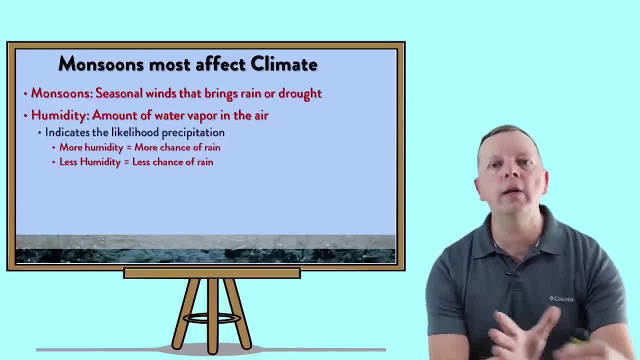 with how the winds move humidity on and off of the Indian subcontinent. We know that humidity is the amount of water vapor in the air And we know that if there is more humidity, there's more chance of rain. There is less humidity. 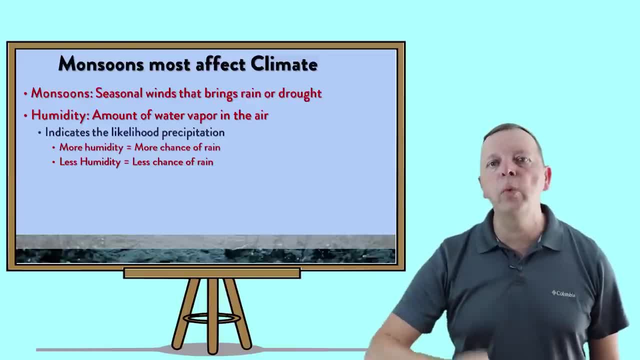 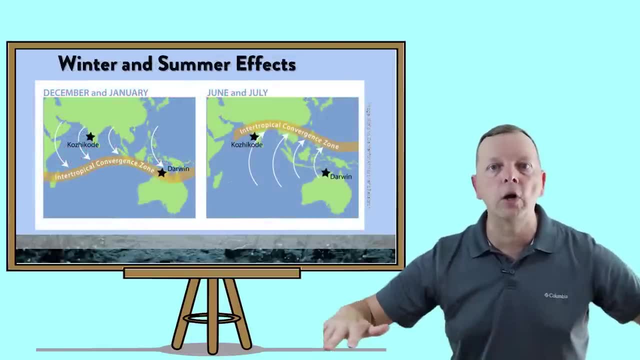 There's less chance of a rain. And what moves these winds is our friend, the intertropical convergence zone. Remember this- is this low pressure cell that is usually along the equator. However, we know that in many different places in the world that the itch. 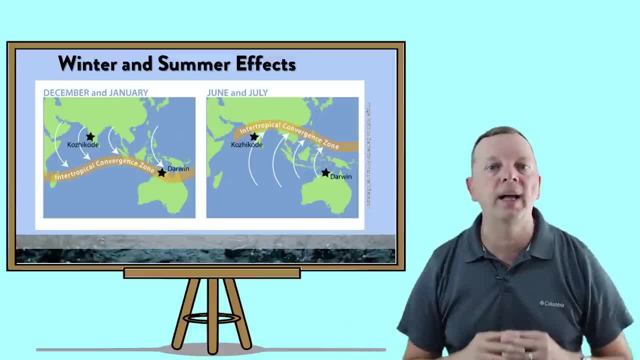 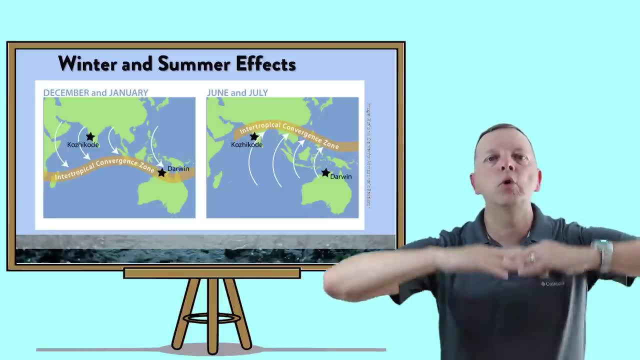 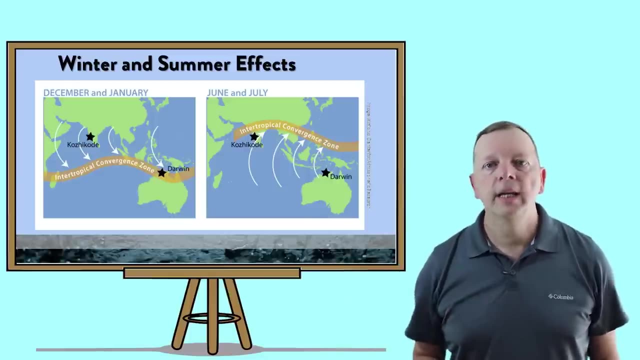 the intertropical convergence zone moves north and south based upon these seasons, And nowhere has as much migration than in South Asia, where the itch will move as much as 40 degrees latitude between summer and winter. Now, what this means is is that when you have the itch all the way down to the south, 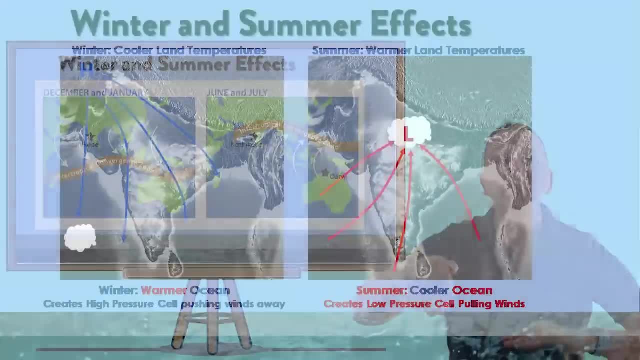 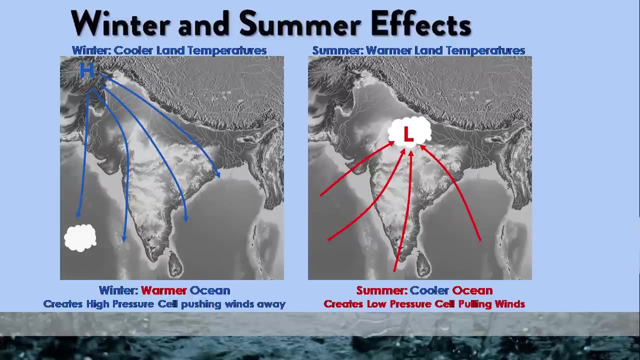 you have that dry air of the satellite cells now moving the northern portion of India And what that does is it has, is winds are pushing all the humidity off of the continent And therefore it doesn't have very much rain. Now what happens in the summer is the itch moves all the way up to the northern. 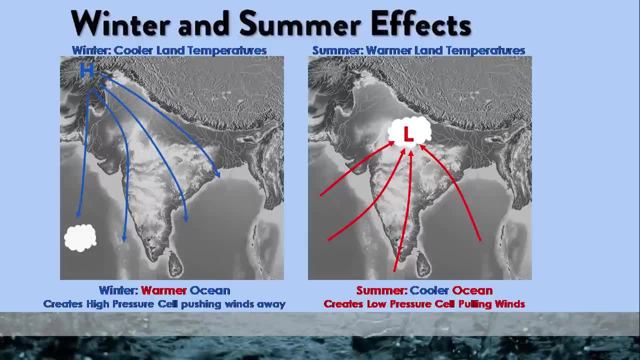 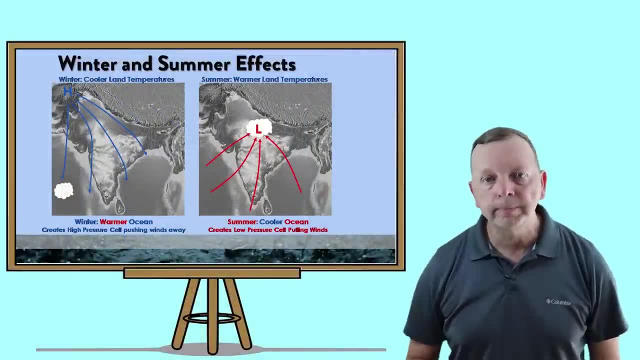 portion of India which have a low pressure cell. Now, low pressure, So we know, brings lots of winds onto the subcontinent, bringing lots and lots of rains. Now, the impacts of these monsoons are pretty striking when we're depending upon whether it's summer or it's winter and summer. 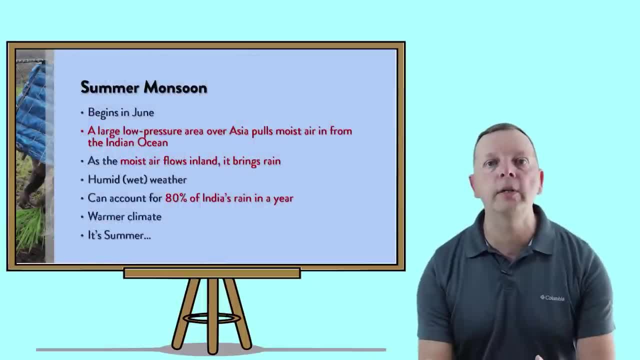 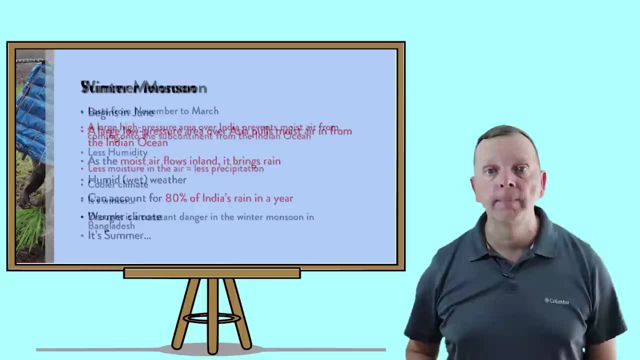 Remember you have that low pressure cells bring all the winds and this humidity on. This is where India gets 80 percent of its precipitation during the summer monsoons. in the winter monsoons, however, because you have a high pressure cell, that is blowing, 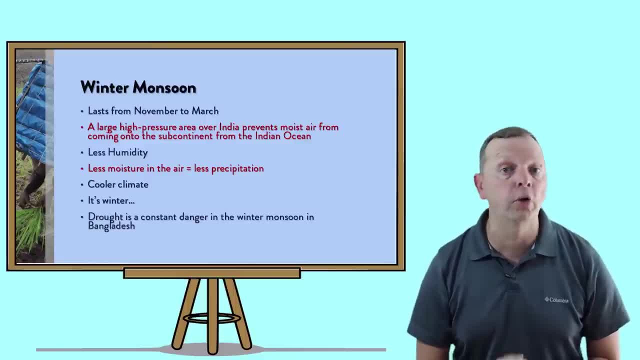 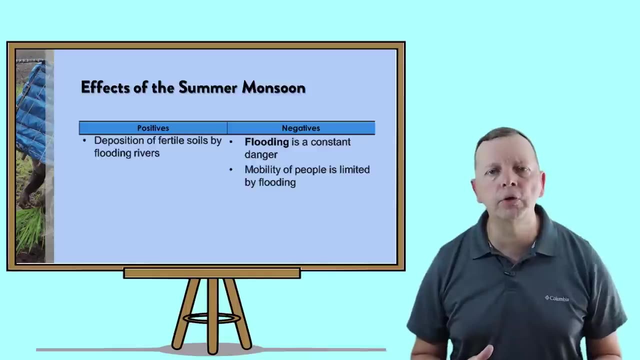 all this precipitation away. Now you have less moisture, less humidity and less precipitation. In fact, drought is a constant problem, especially in areas that are part of this monsoon air region, such as Bangladesh. Now the effects of the summer monsoon. there is a positive, which is you have 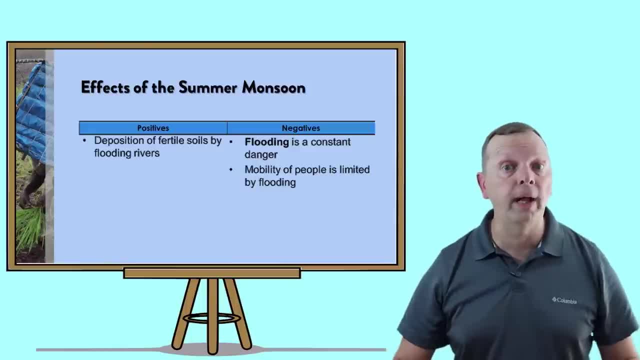 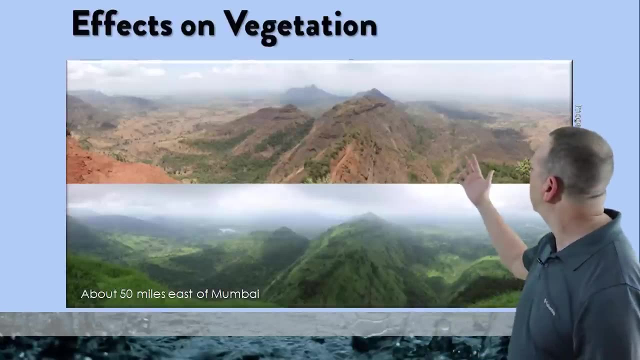 these fertile soils that are deposited, these alluvial plains there during the flooding rivers. But during the summer, you have also the problems of flooding causing a loss, of property damage, as well as interfering with transportation. Now, if you look at this picture here, it's a picture is a one is of the winter. 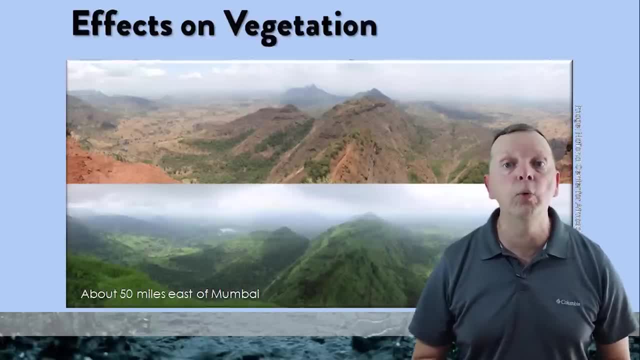 and one is the summer at the same location. Can you determine which ones at summer and which ones at winter? All right, if you said the bottom one is summer, you're absolutely right. This is the effect that happens between the monsoons. 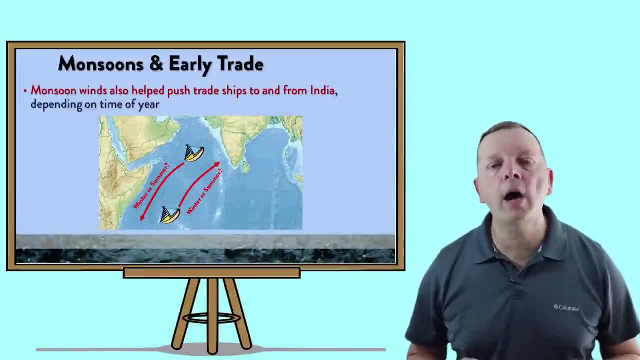 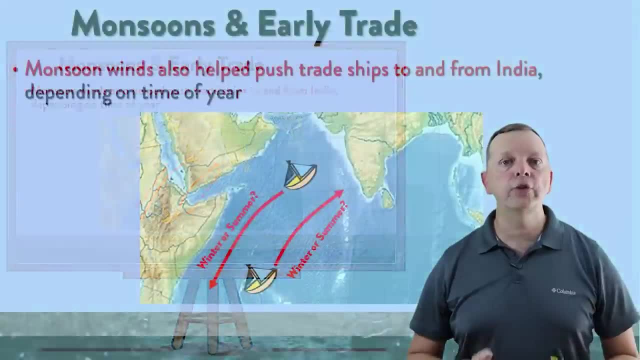 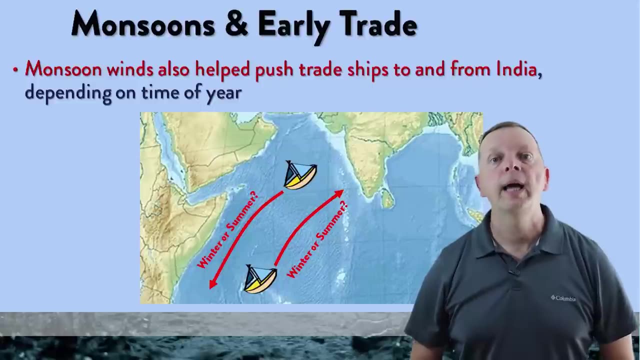 The other thing that monsoons do, in addition to climate, is how it actually impacted trade. So, understanding these monsoon winds, sailors would actually time their journey so that they would be approaching India in the summer, when you have the winds at their back pushing you there. and then their departure from India. 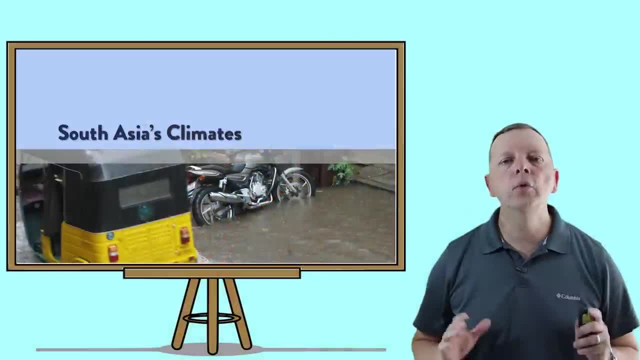 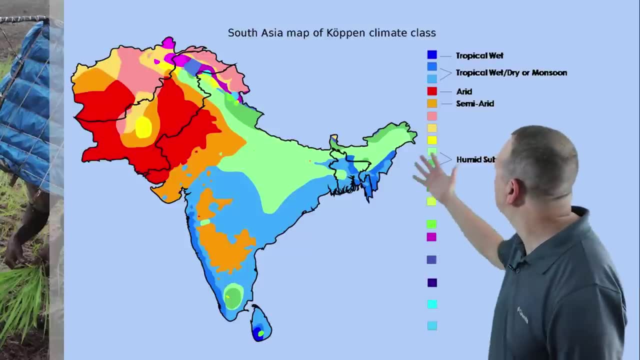 in the winter, when you had their winds pushing you away. So now we understand the importance of monsoons, We can start looking at the actual climates of Southeast Asia, and they're depicted like that. Now there actually is four major climate types which we're going. 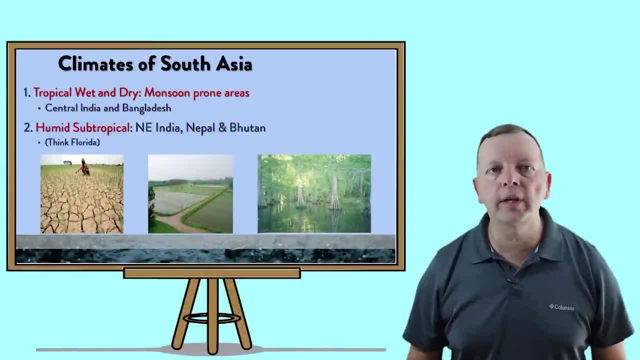 to talk about, and we can break those up by region. Now, the first climate we have is your tropical, wet, dry, And here we're going to find that type of climate in those areas of South Asia that are more impacted by these monsoons. 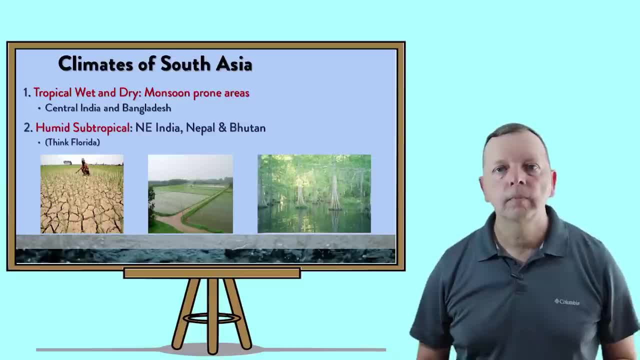 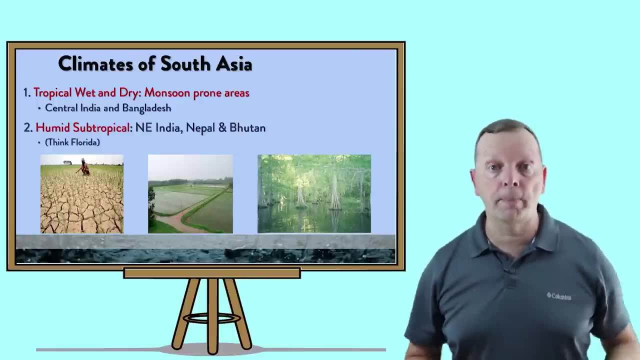 That would be central India and Bangladesh. Now, as you go up to the northeast portion of India, Nepal and Bhutan, you start getting into a humid subtropical climate. This is much like what we find in Florida or even here in Bryan, Texas. 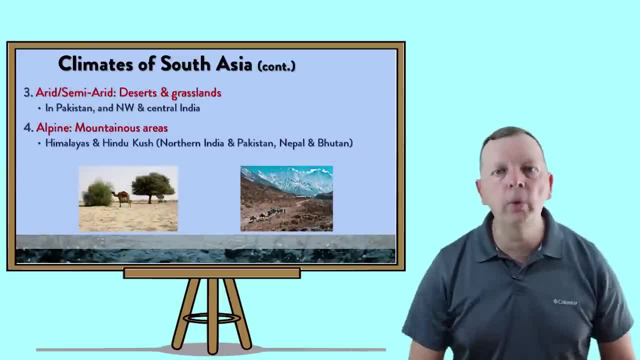 And the third climate we have. really there's two. You have your arid and your semi-arid deserts and grasslands We have in Pakistan and northwest India. you have the Thar Desert in it, And then you also have in central India. 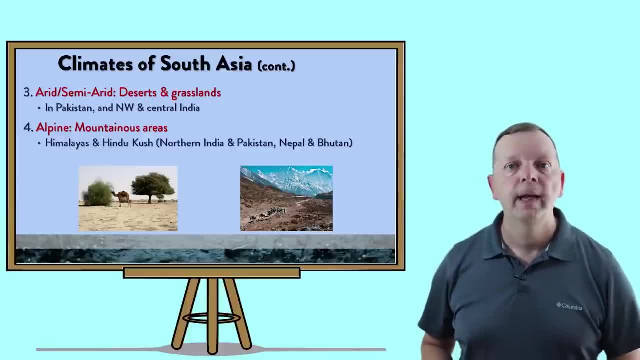 you have the Deccan Plateau, which is a semi-arid region, And then if you have the tallest mountains in the world, you're going to have your alpine or your highland climates, And here we have all those along the Himalayas and the Hindu Kush found. 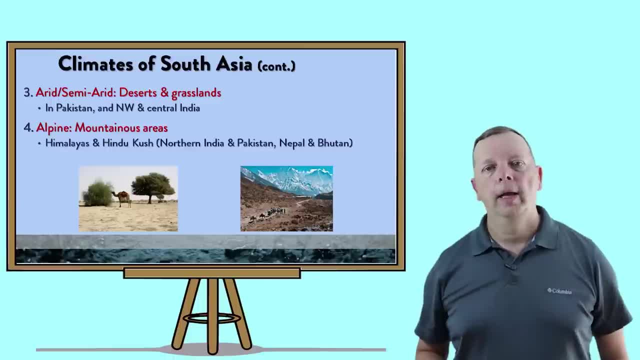 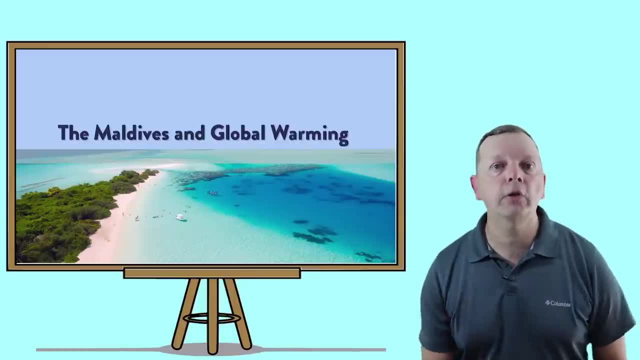 in the northern portion of India, Pakistan, Nepal and Bhutan. All right, So those are the most important climate types we have in South Asia. Now, if we're going to talk about climate, one of those conversations that often comes up is that of global warming or climate change. 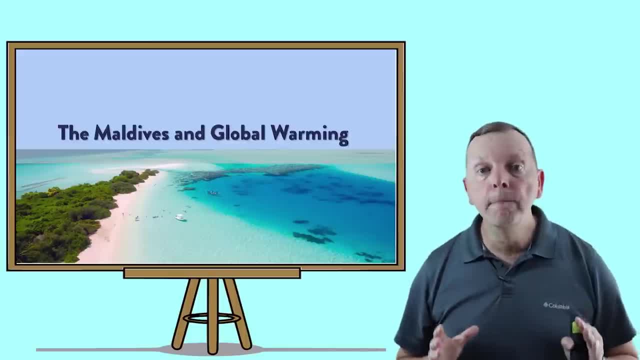 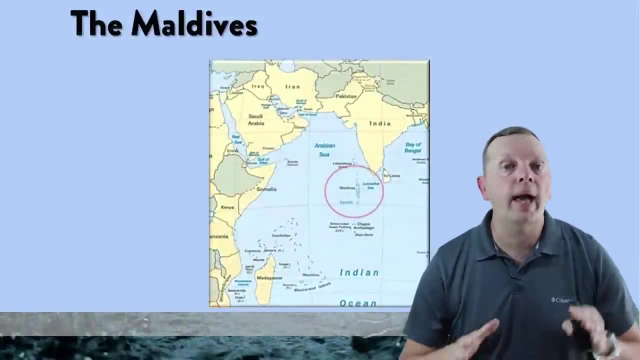 And nowhere is probably has the potential of being more impacted than the Maldives. Remember we talked about the Maldives when our country is very quick. This is that group of islands off to the southwest portion of India. It is known as an archipelago. 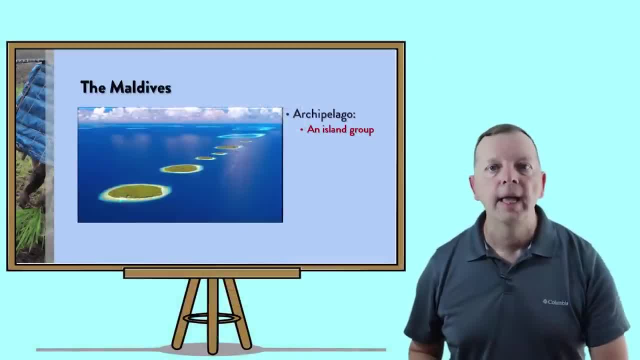 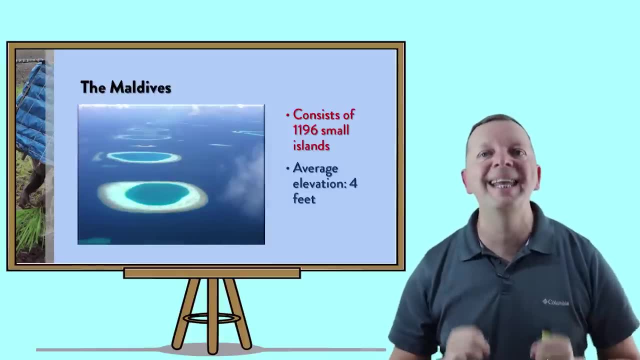 An archipelago is a group of islands And we talk about a group of islands. We know that there's lots of islands. In fact, there is over eleven hundred and ninety six small islands, and they're not very big at all, nor are they very tall. 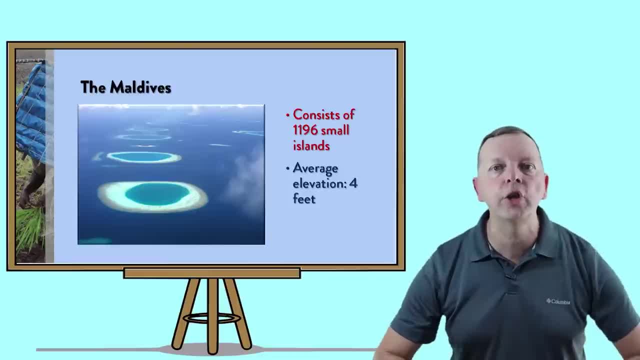 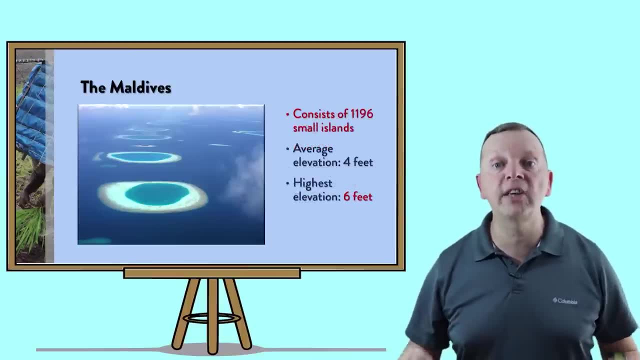 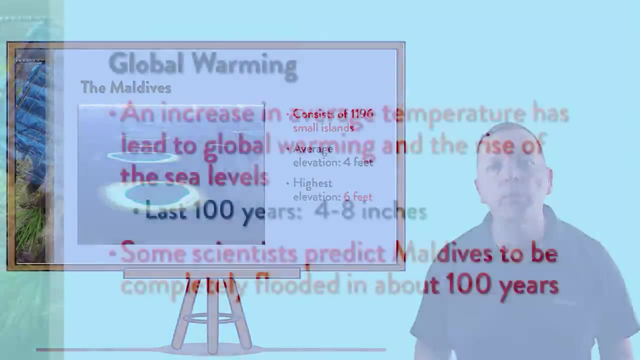 The average elevation of the Maldives is about four feet above sea level. In fact, the tallest point in the Maldives is just six feet tall. That is just about like here is not very tall at all. So the problem with that is that there is 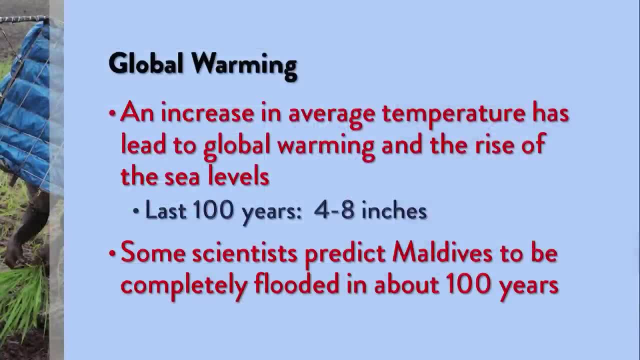 lots of scientists who believe that what is happening is because of global warming. we have the rise of sea levels. in fact, it's been measured that in the last hundred years is actually the seas have raised anywhere between four and eight inches. That doesn't seem like a lot. 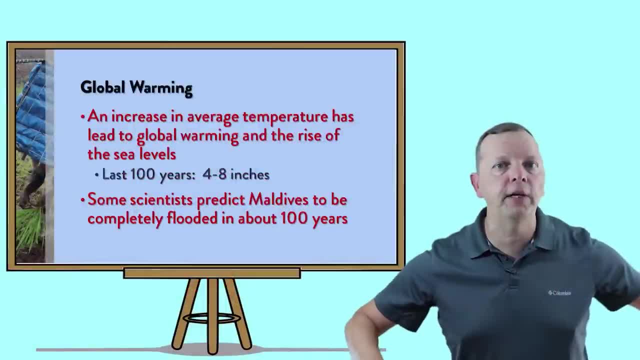 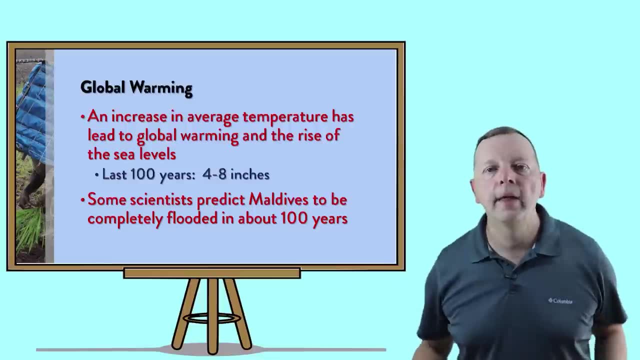 But when your country's average elevation is just four feet tall, well, this is pretty important. In fact, some scientists believe that, due to global warming and the rising of the seas, the Maldives will be completely covered in the next hundred years. 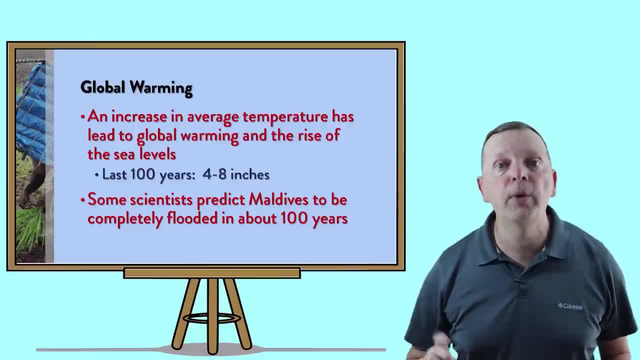 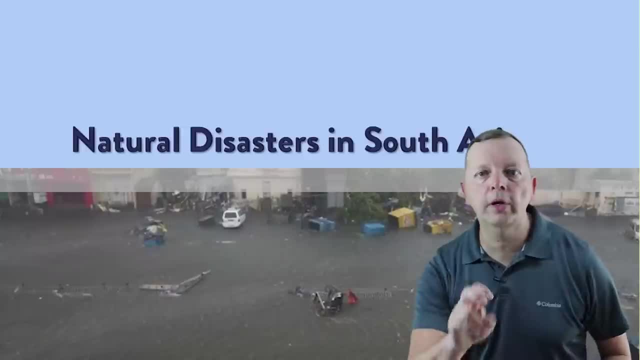 And some believe it will actually be uninhabitable within 50 years. All right. so if that's not enough of a natural disaster, there are others. We're going to talk about two. The first are cyclones. Now remember, we talk about hurricanes. 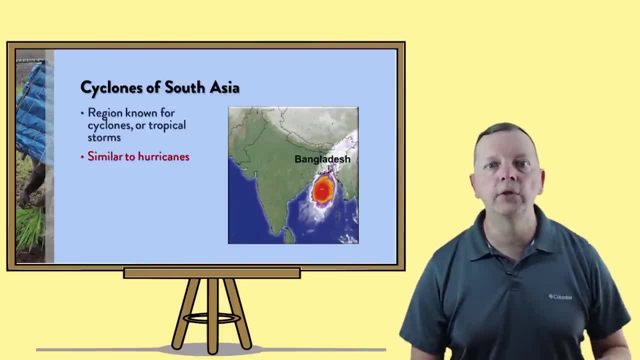 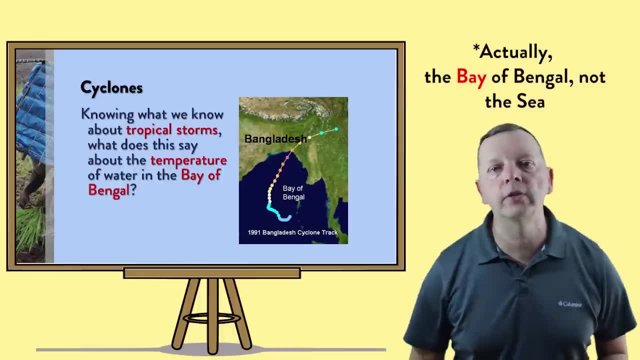 Guess what a cyclone is? A cyclone is a hurricane, It's a tropical storm, And we find these largely going into the sea which is known as the Sea of Bengal and striking into Bangladesh. But not all of our natural disasters are against climate.